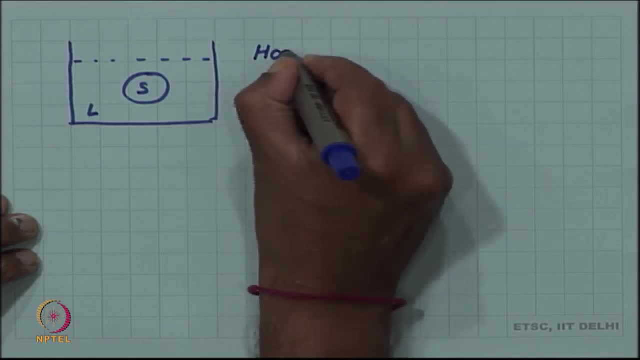 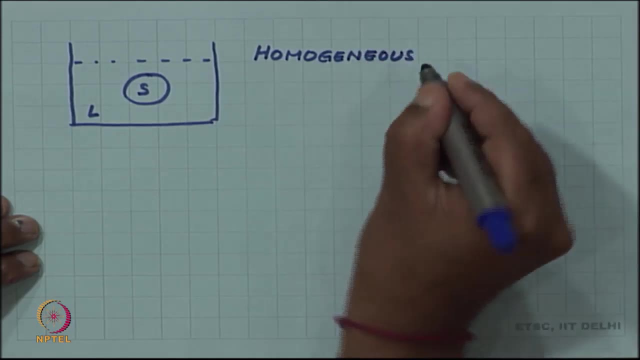 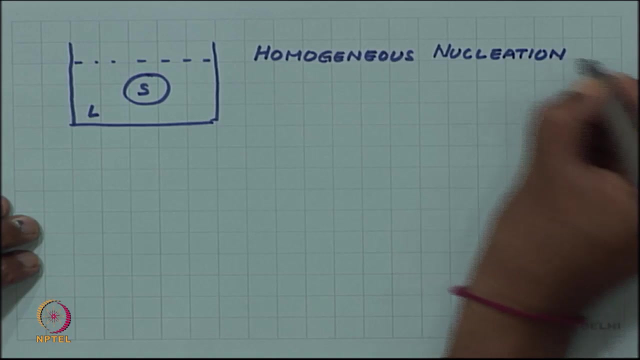 This is an example of homogeneous nucleation. So what we have been discussing till now is like the formation of a solid nucleus inside a liquid. This is an example of homogeneous nucleation. We did not use this adjective before, We were simply calling it nucleation, but this is 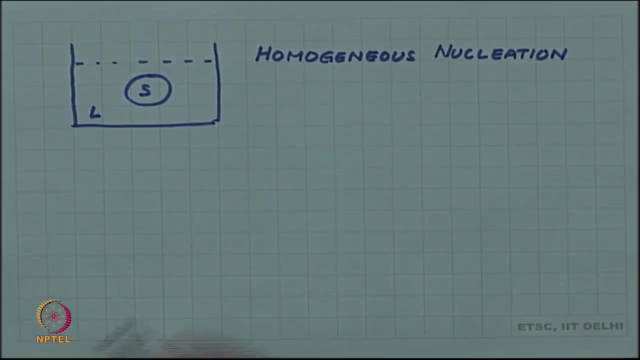 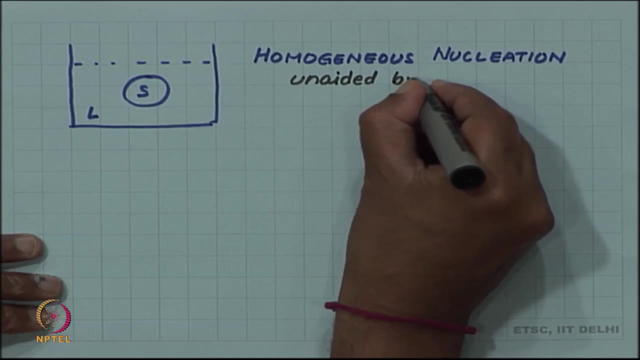 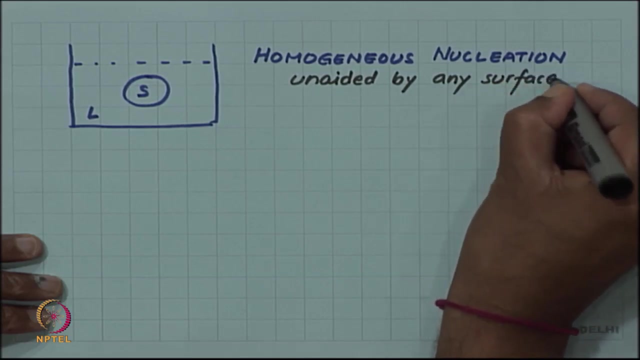 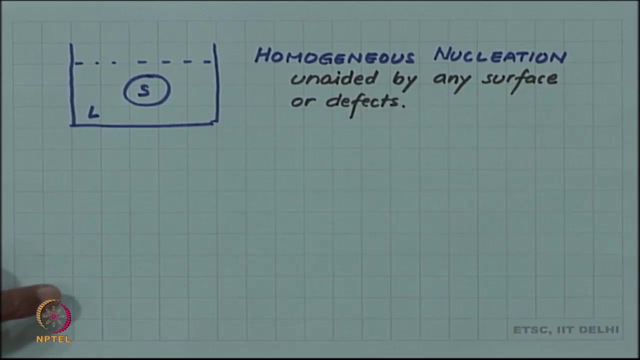 an example of homogeneous nucleation, which essentially means a nucleation unaided by any surface. So we have the process of nucleation or deformation, or defects. We took this up because it is mathematically simpler to analyze. However, in reality this is a quite unlikely situation. 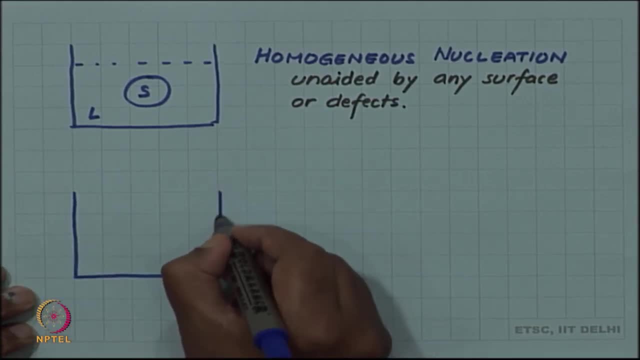 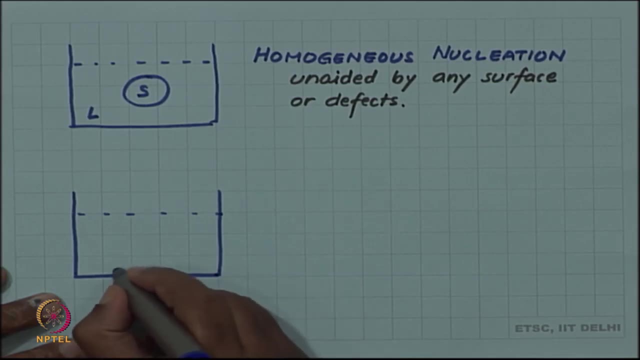 A more likely situation for nucleation to happen, particularly in the case of freezing, is that nucleation will happen at the container wall. So that is the first point. The second point is that we want to have the case of a solid, So the solid may form at the wall of the container. this kind of nucleation is called 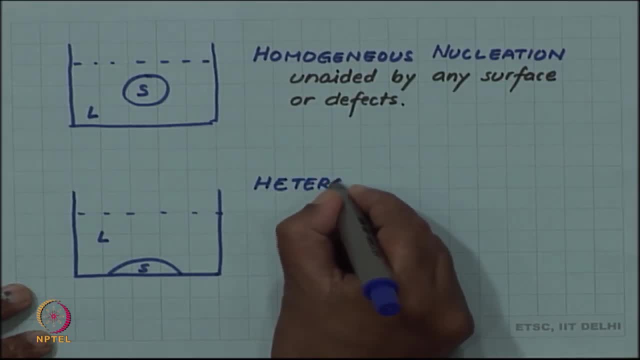 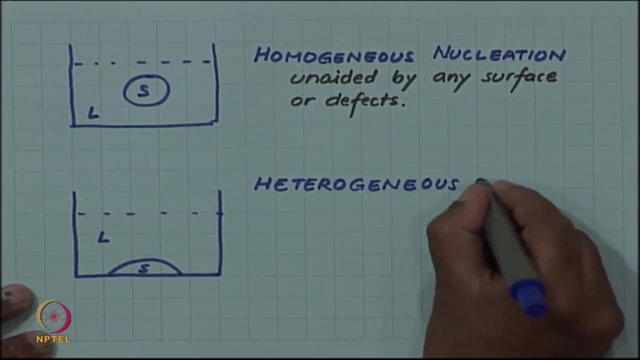 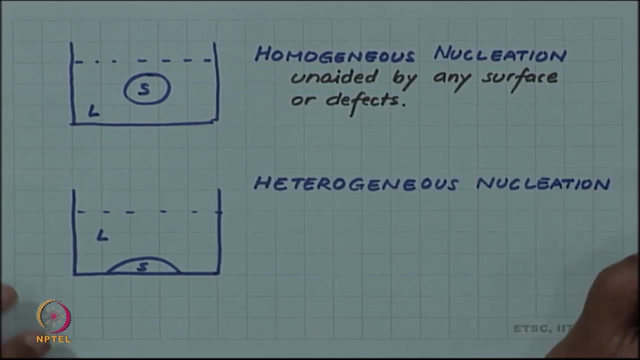 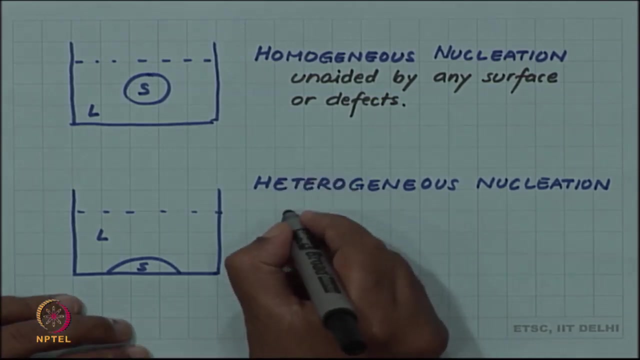 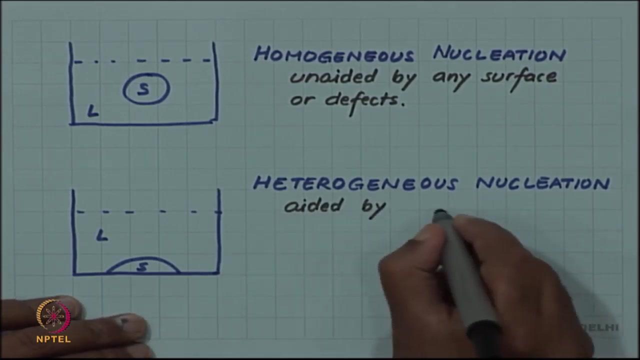 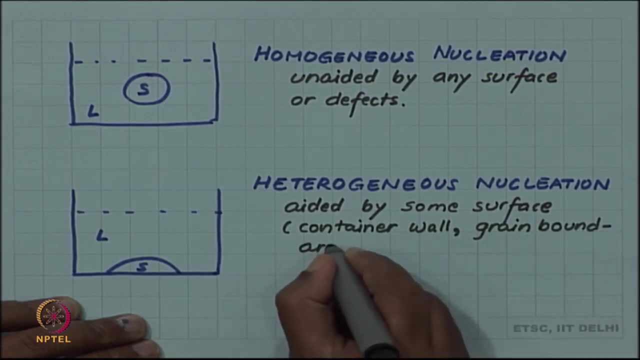 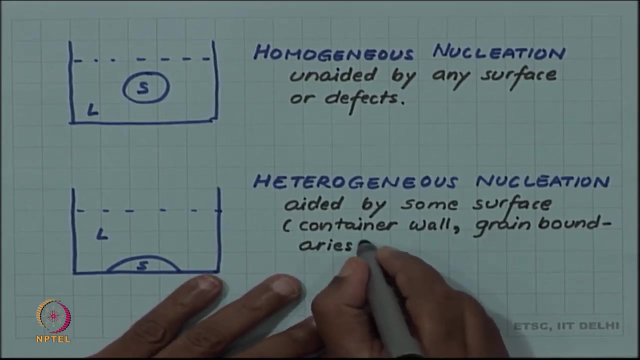 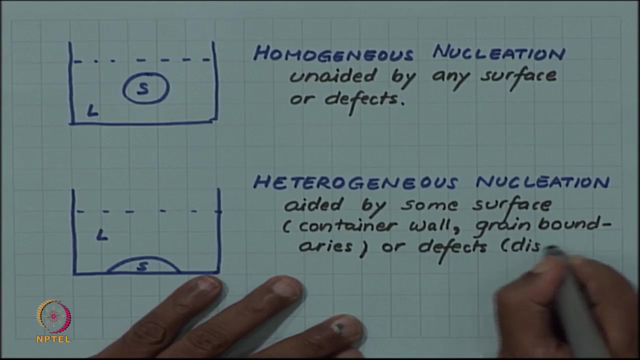 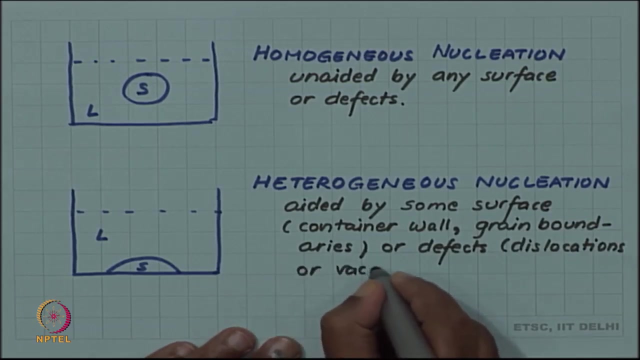 heterogeneous nucleation. heterogeneous nucleation: This kind of nucleation is aided by by some surface, For example, like in this example, container wall, or in case of solids, it can be grain boundaries, or it can be other defects such as dislocations, or it can be other defects such as dislocations. 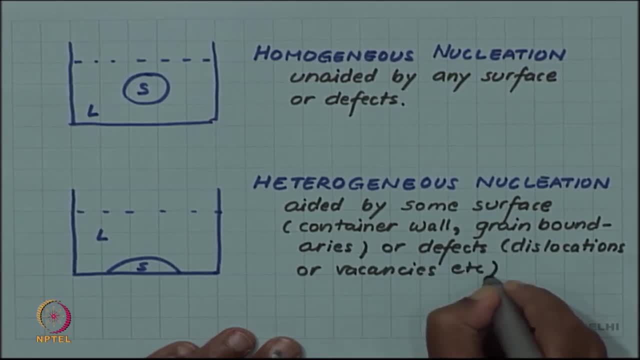 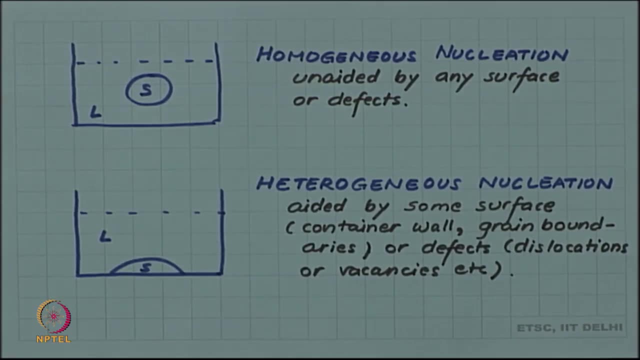 So this kind of nucleation is called heterogeneous nucleation and it is a more common kind of nucleation. mostly, for example in this situation or itself, you can see, in case of solidification it is quite likely that nucleus will form at the container wall rather than totally. 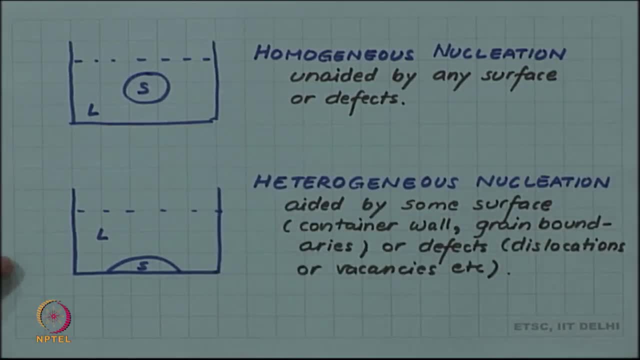 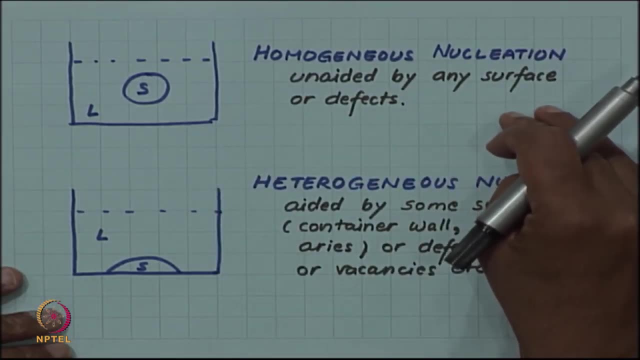 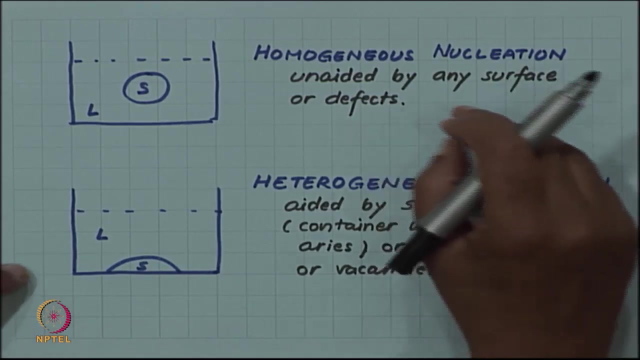 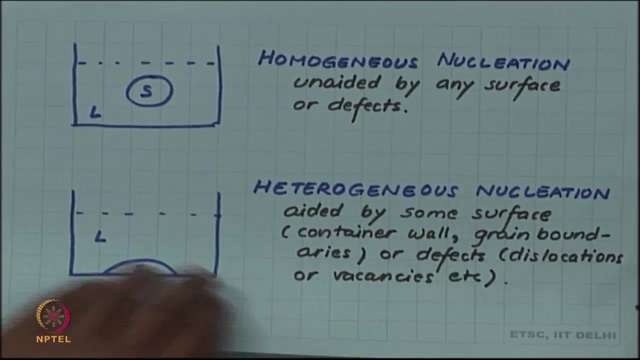 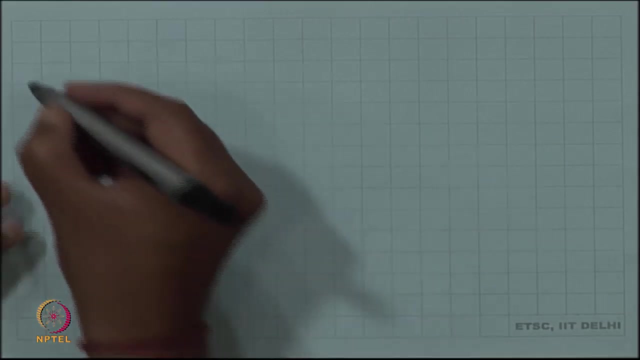 inside the liquid. So homogeneous nucleation is a nice, simple situation, easy to analyze mathematically and in a study in laboratory situations can be created such that we have homogeneous nucleation, but most practical nucleation situations are heterogeneous nucleation. So let us look at heterogeneous nucleation in little bit detail, Just like we analyze. 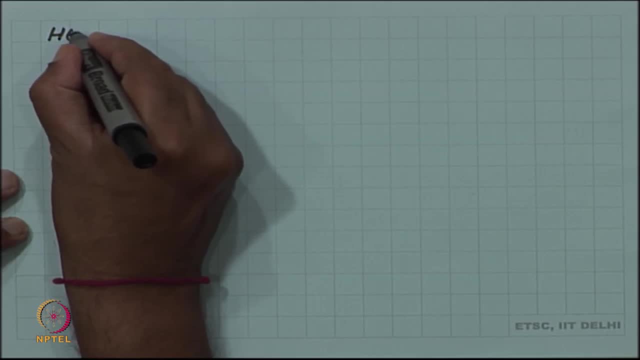 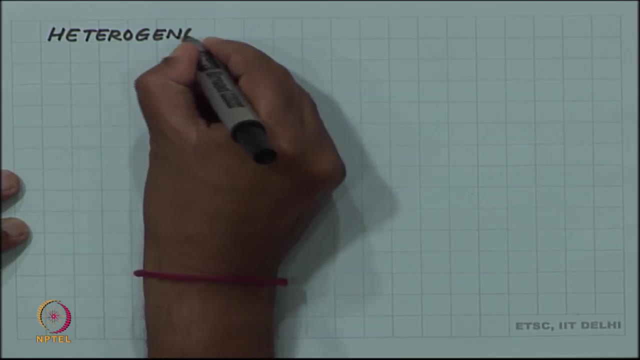 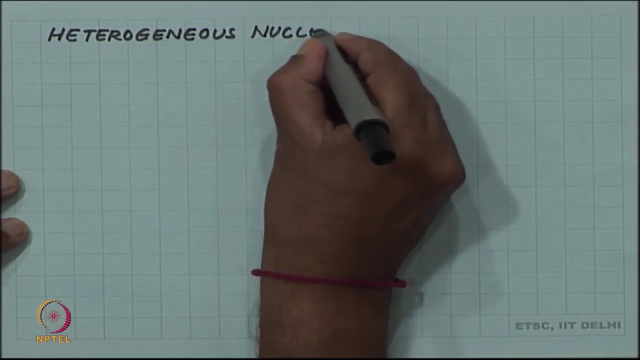 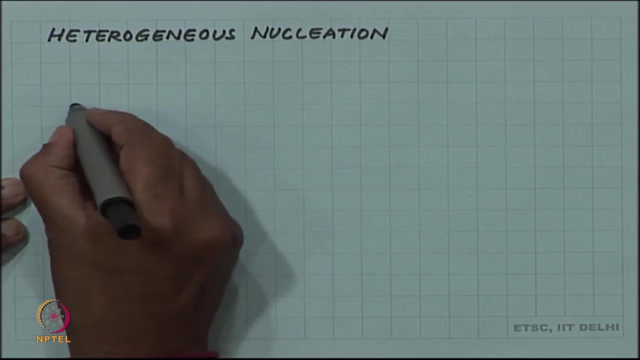 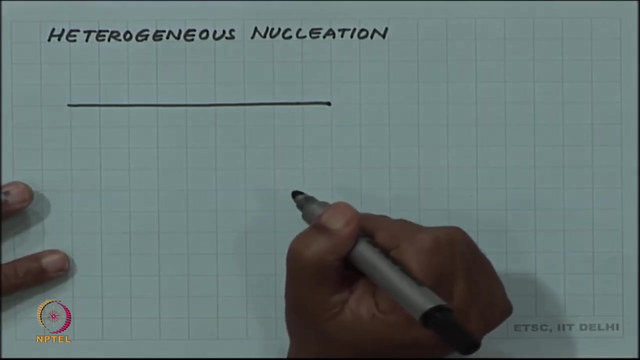 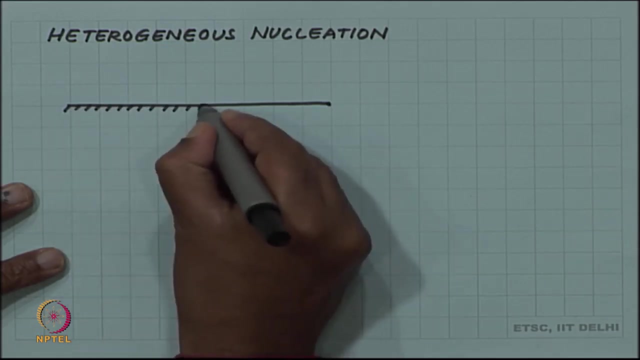 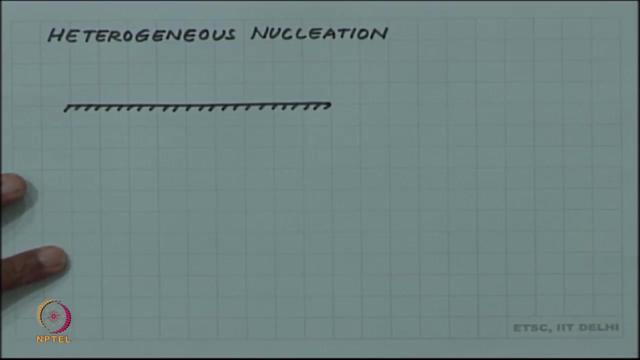 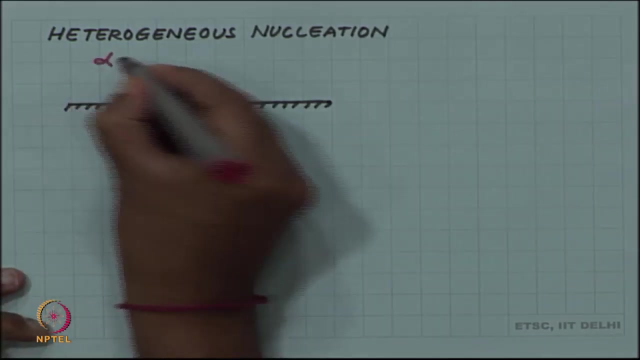 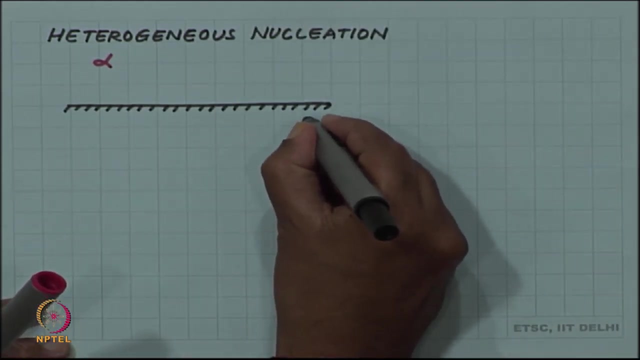 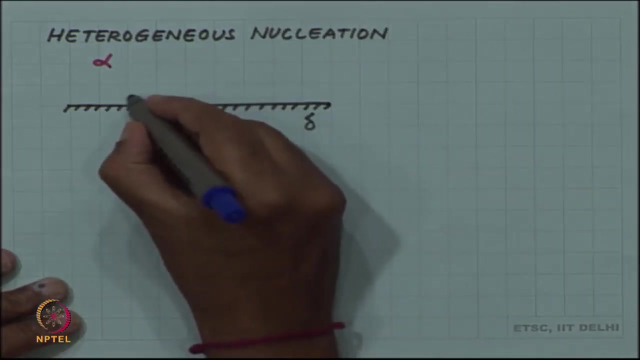 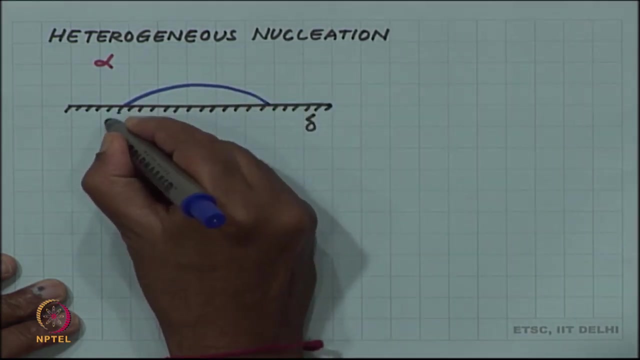 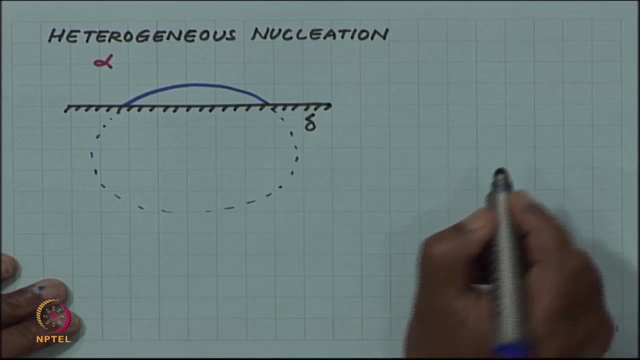 it homogenous nucleation in terms of energy. let us do a similar analysis for heterogeneous nucleation. So let me assume some sort of container, wall, ball or substrate over which there is some phase, some phase alpha, and let me call the substrate itself delta, And in alpha a nucleus of beta forms alpha. 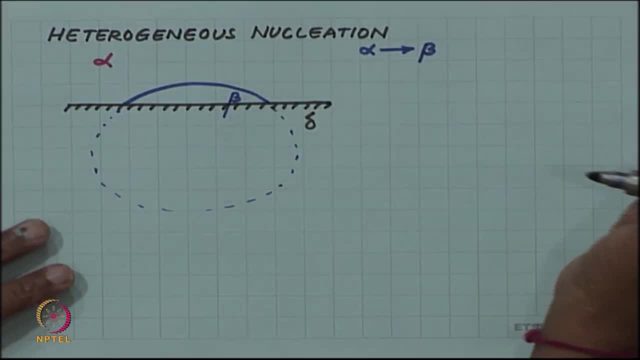 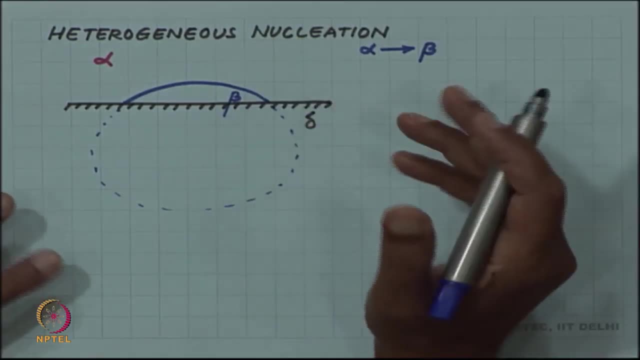 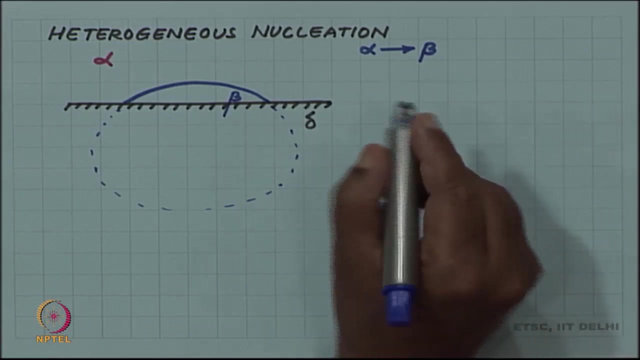 is transforming in beta On this surface of delta. So that is why it is a heterogeneous nucleation and, in particular, again, just like we simplified the geometry of the problem in homogeneous nucleation by considering a spherical nucleus, Here again we are simplifying the geometry by considering: 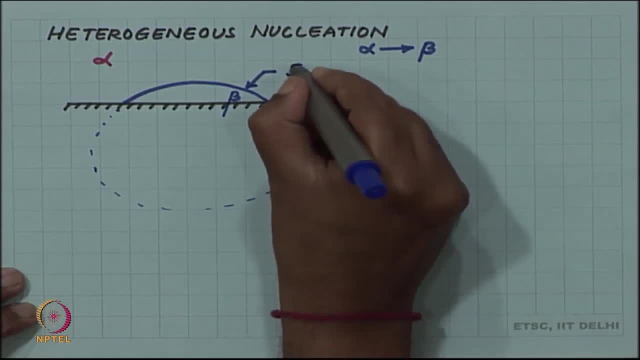 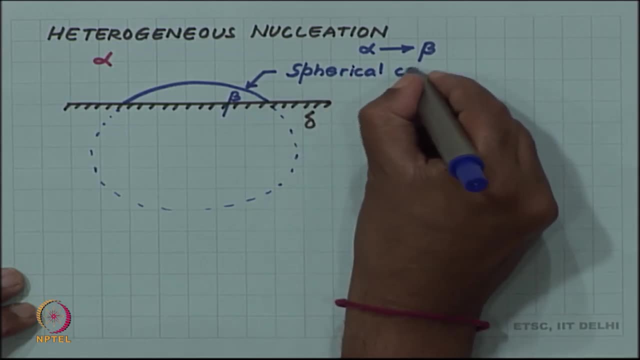 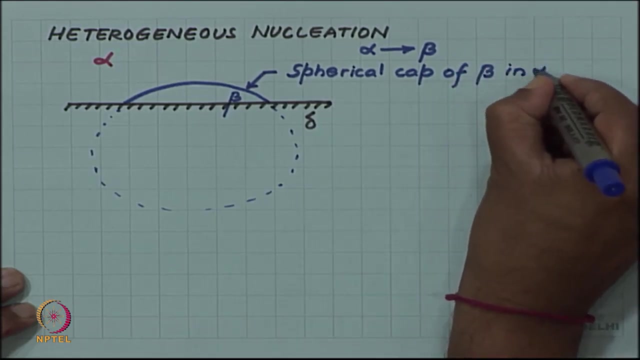 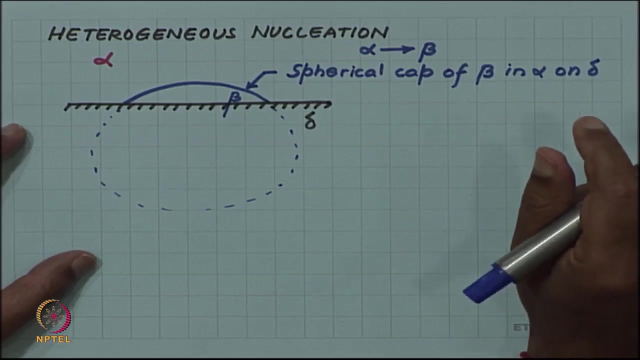 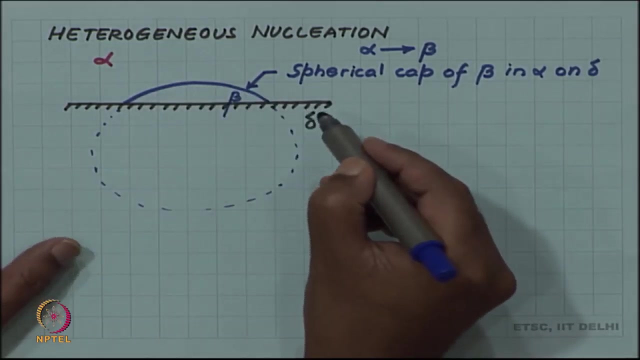 a spherical cap nucleus. So essentially we are saying that beta is forming as a spherical cap of beta in alpha on delta. So we by spherical cap I mean that this surface, the alpha beta surface, is spherical, and I have tried to draw the entire sphere here So you can see that. 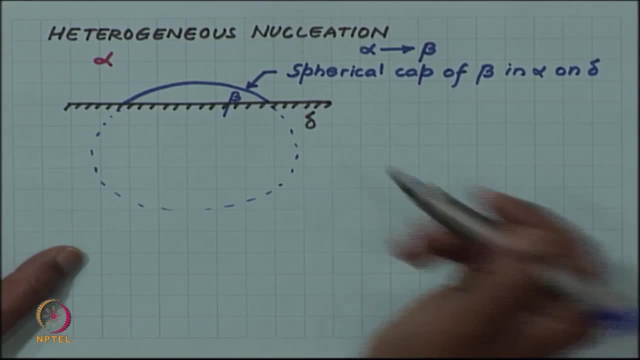 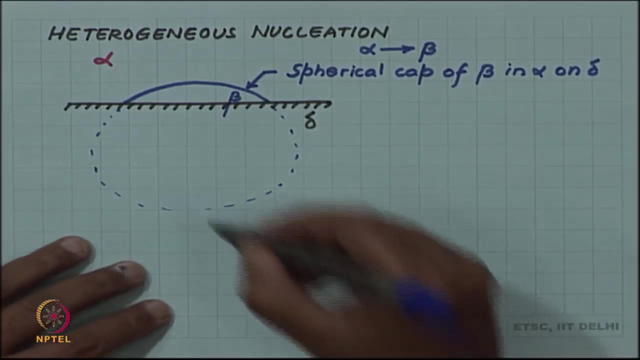 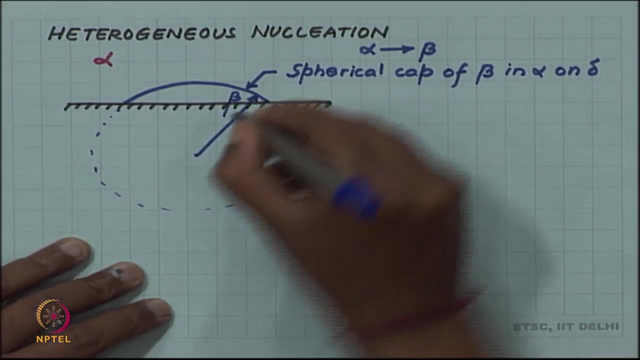 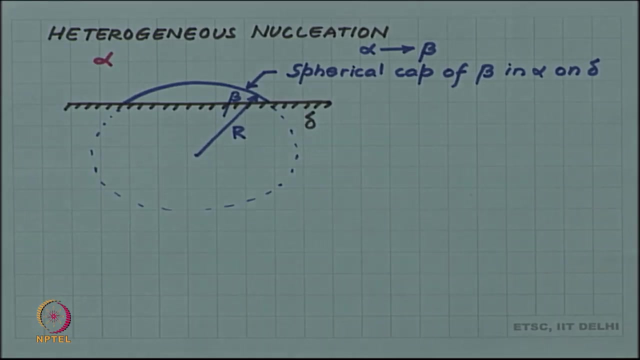 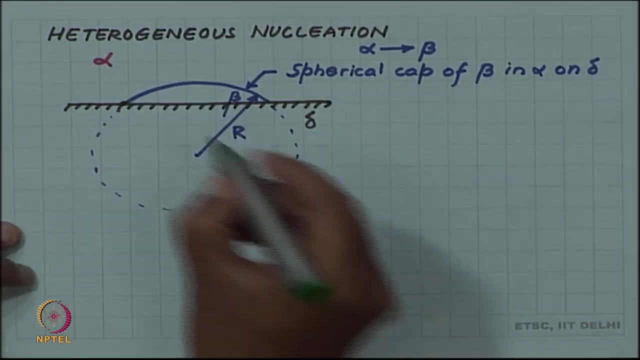 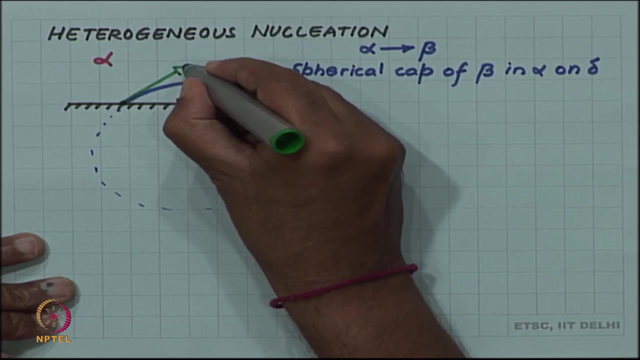 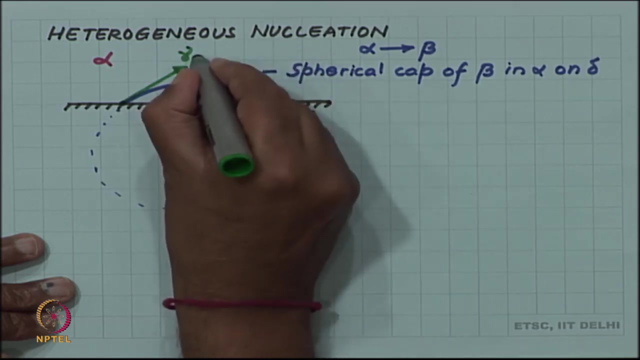 this is sphere. So you have, for example, the alpha beta interface and I am showing the surface tensions by these arrows. So this is gamma alpha beta and this is another surface between beta and delta. So this I write as gamma beta, delta. 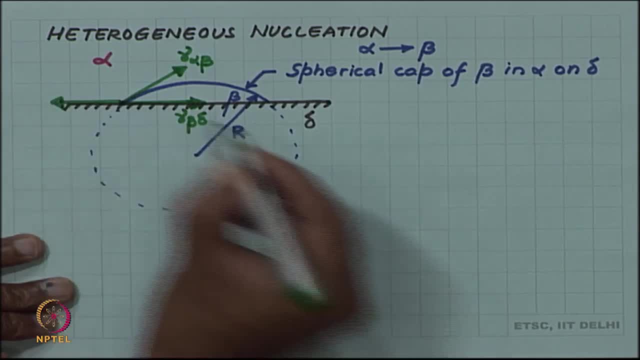 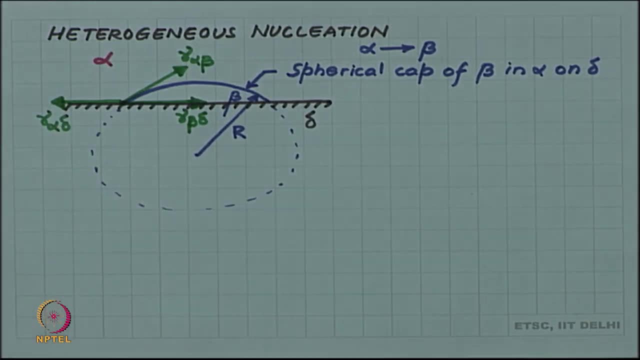 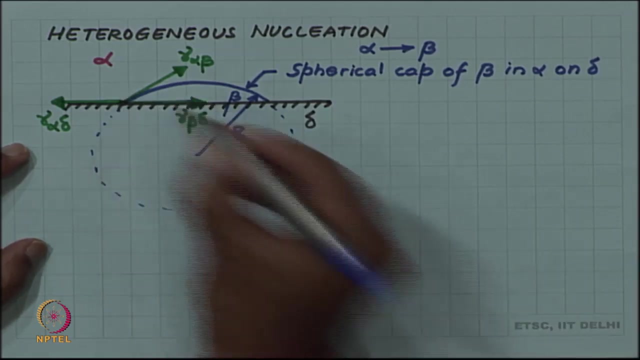 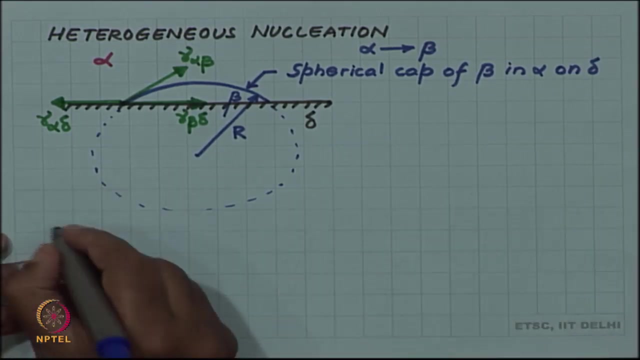 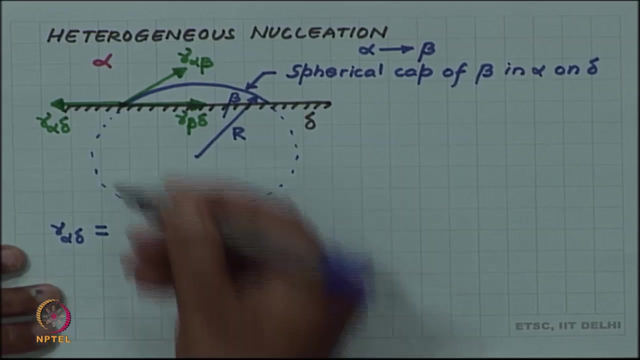 And you have a surface between alpha and delta which I write as gamma alpha delta. Since these 3, these 3 surface tensions are locally in balance, at this point we can write an equilibrium condition For these surface energies in terms of gamma alpha delta. if I take the horizontal component, 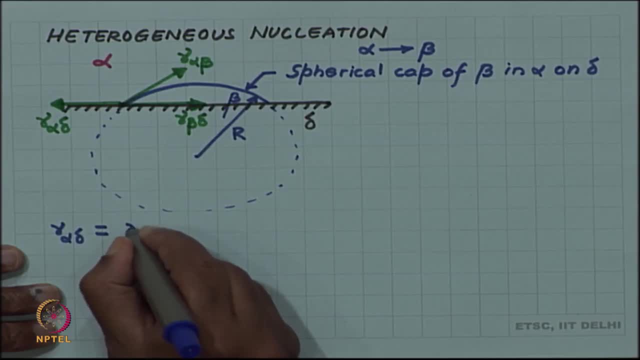 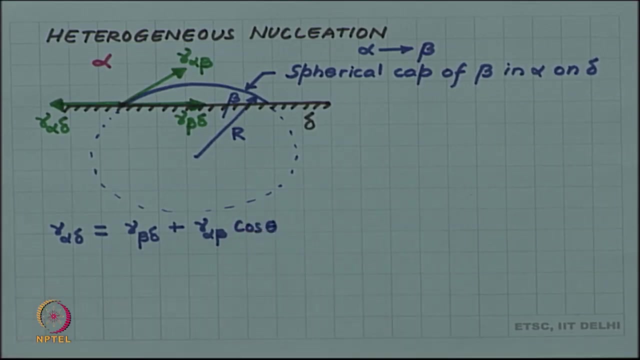 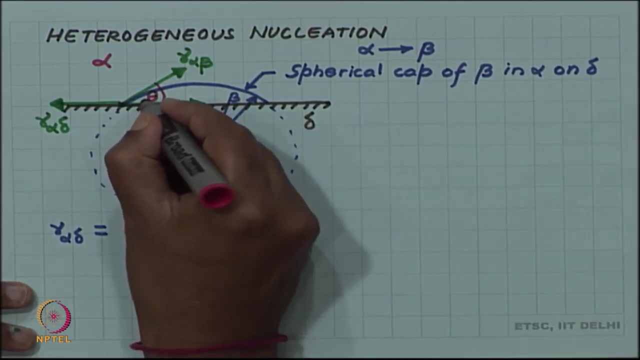 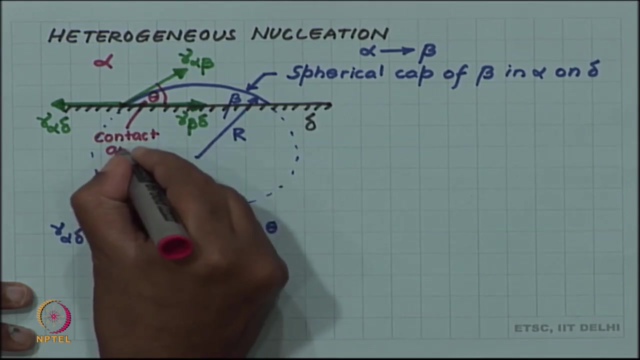 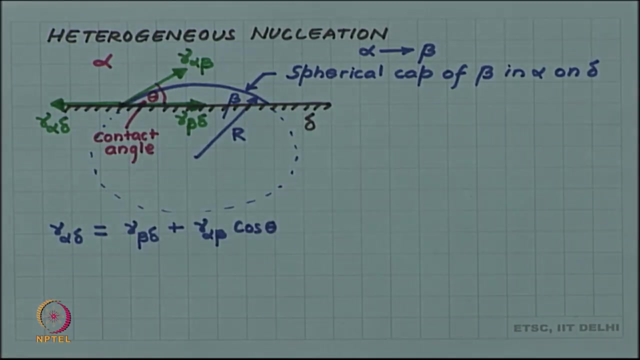 then gamma alpha delta will be equal to gamma beta delta plus gamma alpha beta cos theta, Where theta is. this angle here also known as the contact angle, 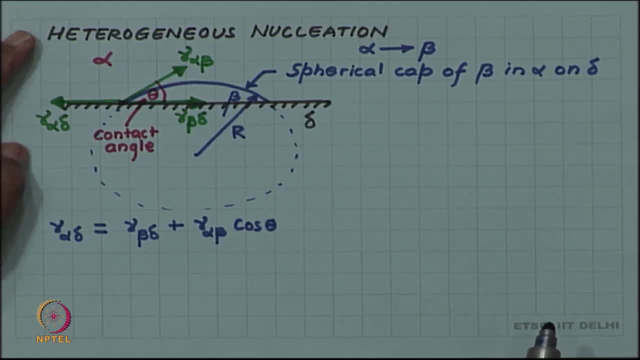 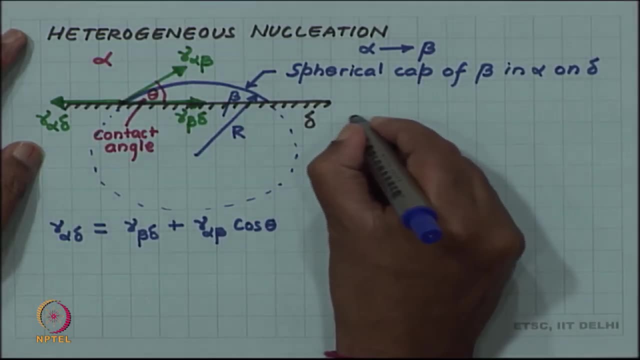 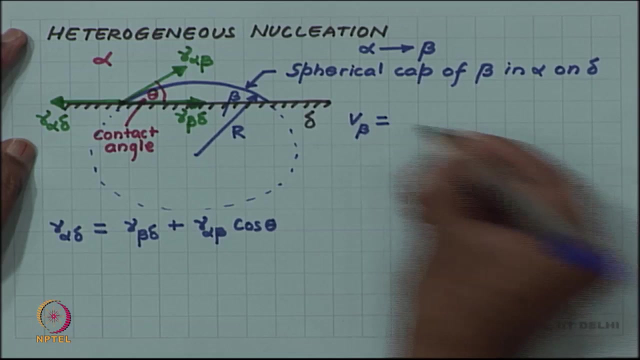 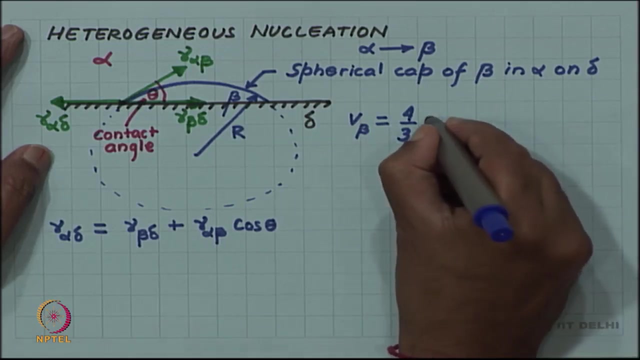 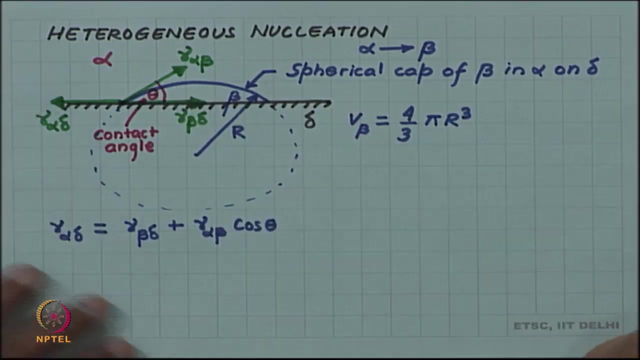 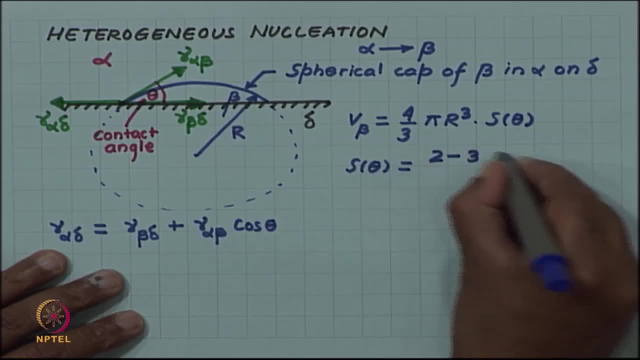 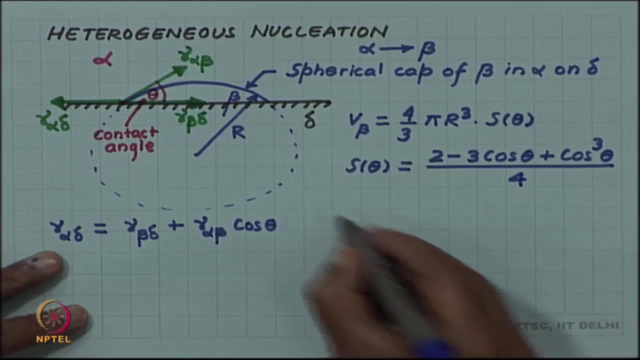 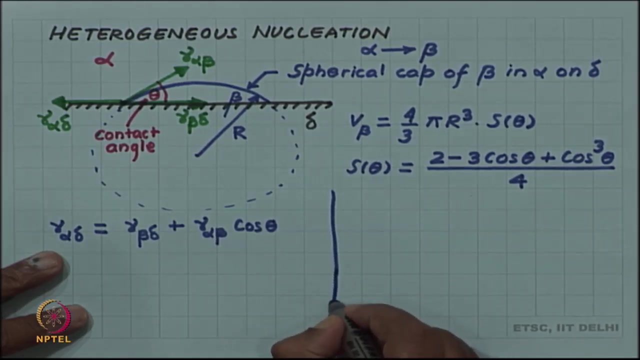 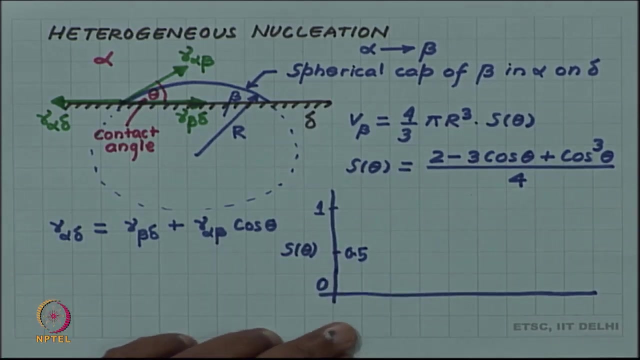 2 minus 3 cos theta plus cos cube theta by 4. function. So let us plot S theta: this is 1, this is 0.5 and this is 0. So this is 0 and the contact angle: theta varies between 0, 280 degree. So if you look at this function, 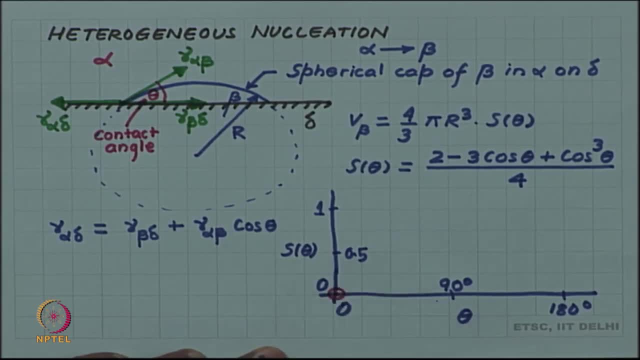 it will be 0 at theta is equal to 0, it will be 0.5 at theta is equal to 90 degree, So it will be 1 at theta is equal to 1 at theta is equal to 180 degree. it will be 1 at theta. 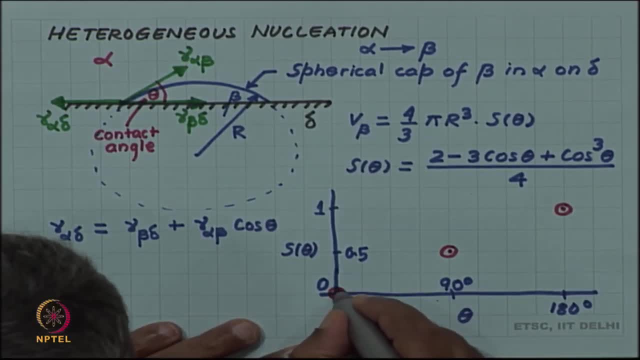 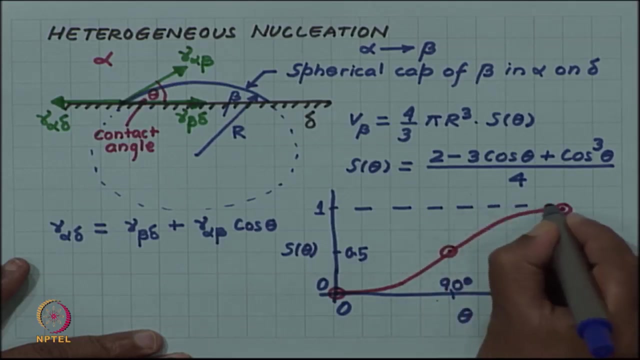 is equal to 180 degree And in between it takes a sigmoidal shape, something like this. So this is 0.5 at theta is equal to 0,. this is 0.5 at theta is equal to 180 degree. So 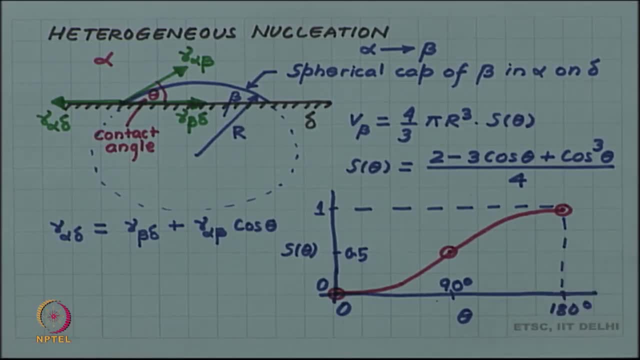 volume of the spherical cap, depending upon the contact angle, can be any fraction of the volume of the full sphere, and that fraction is given by this S? theta which depends upon the contact angle. in this way, We also require the surface area of the spherical cap. 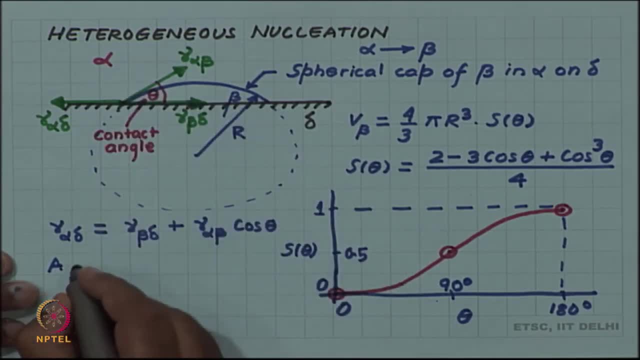 So that is the interface between alpha and beta. So that area I call A alpha beta and that can be shown to be 4 pi r square 1 minus cos theta by 2.. And similarly I require the area between beta and delta. So this is the surface area of the spherical cap. So this: 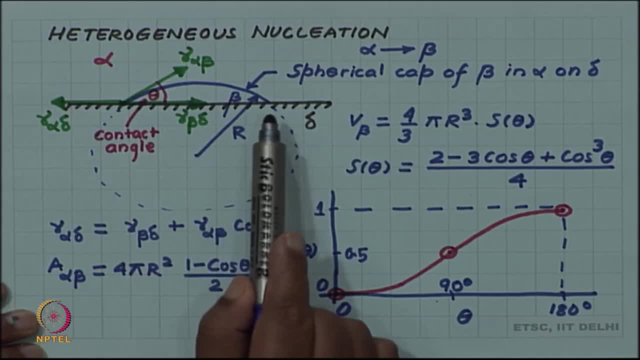 is the surface area of the spherical cap. So this is the surface area of the spherical cap. The surface area is 2 pi r square 1 plus cos theta, and the surface area is 2 pi r square- 2 pi r square Gergan delta. That is the circular base on which thisit is the base, So that 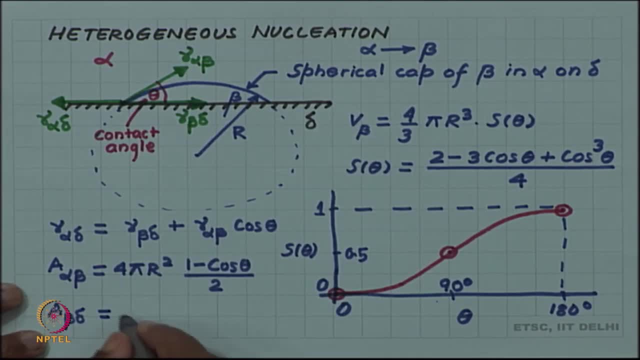 is the base, circular base on which the spherical cap is sitting. so that circular base on which this spherical cap is sitting, A beta delta, its pi r square 1 minus cos square, theta. So we have all the geometrical parameter: the volume of this spherical cap, the crop. 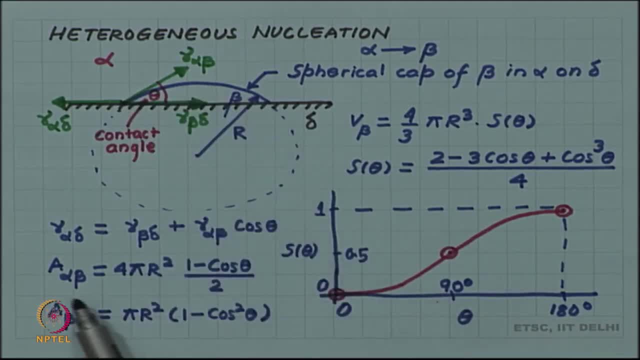 the promise: both parts of the sphere and the surface area it divider by 1.. Ante, VIP, sample your GPA lemons or real. please read and read immediately. I will have these, these two, putting them curved. surface area of the spherical cap: a alpha, beta, and the horizontal base, the circular. 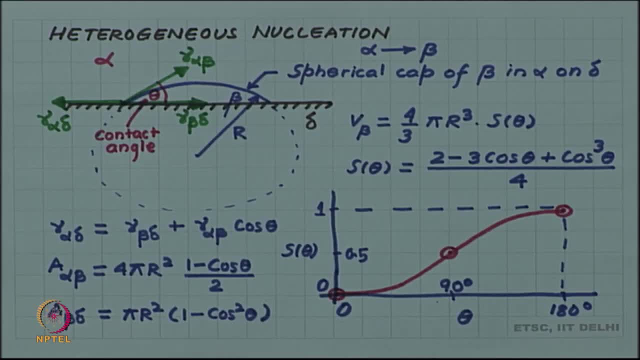 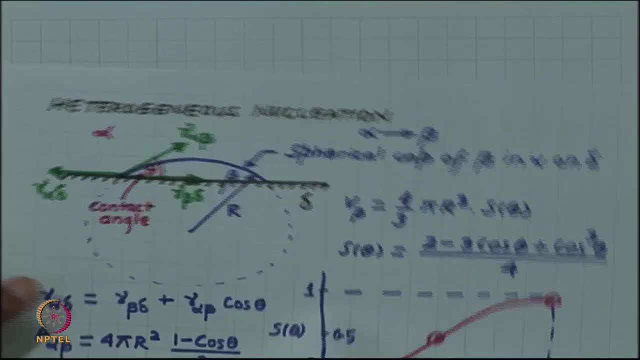 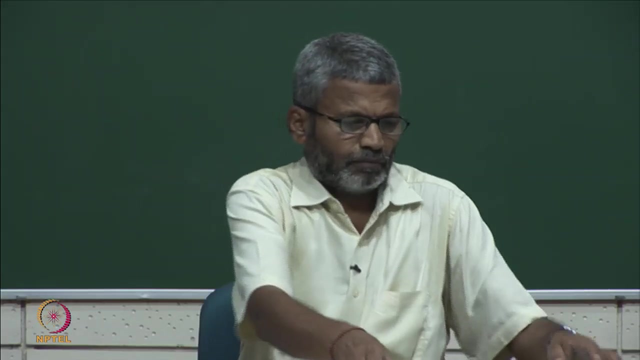 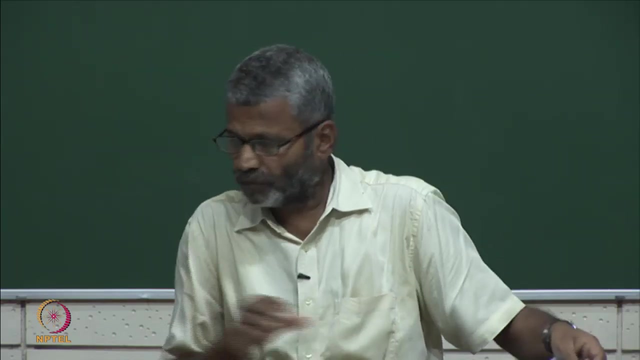 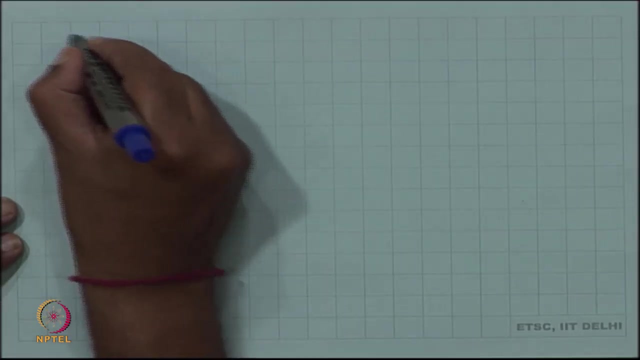 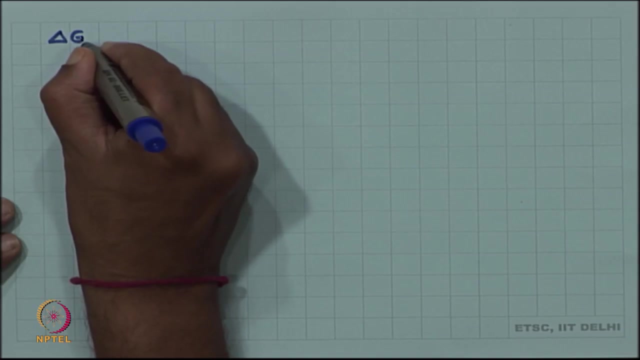 base, a beta delta in terms of r n theta, the radius of the spheric sphere and the contact angle theta. So with this we can take our next step of developing the energetics. So recall that we had, we can write the energy of formation. 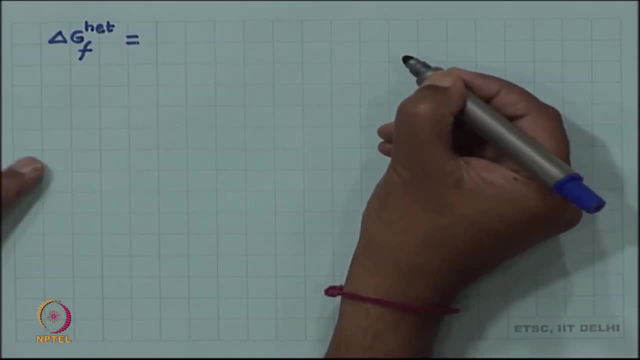 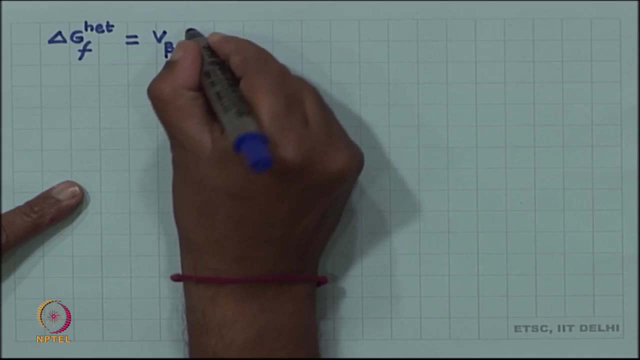 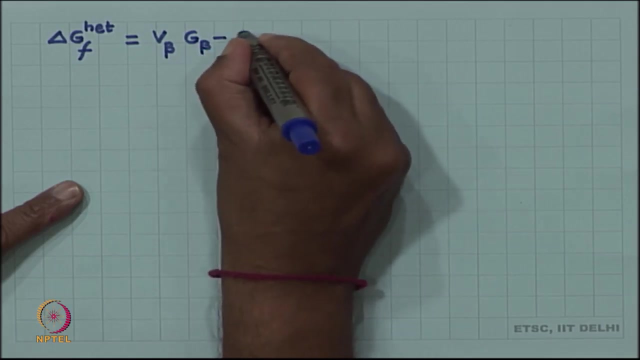 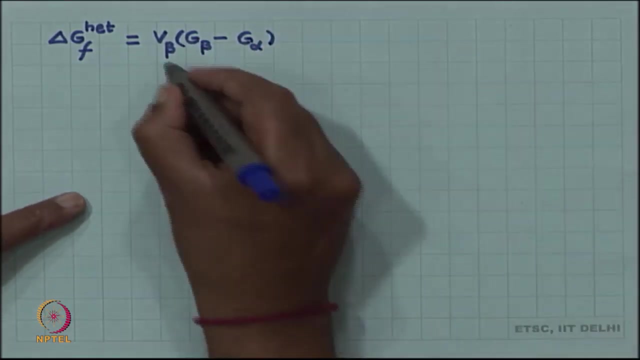 for the heterogeneous nucleation, For the heterogeneous nucleation, For the nucleus, that will be volume of the nucleus, which is V beta times the free energy per unit volume of beta minus the free energy per unit volume of alpha. Again, we are assuming that there is no volume change between beta and alpha, So the same volume of alpha transformed. 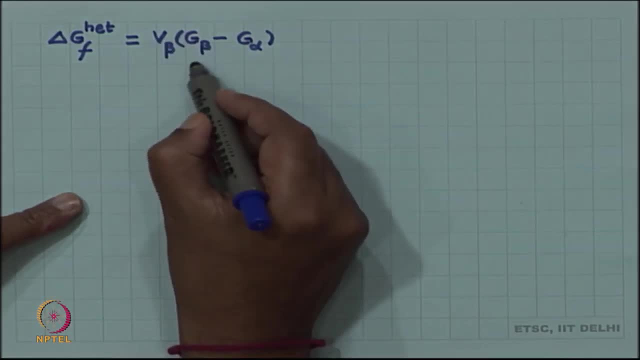 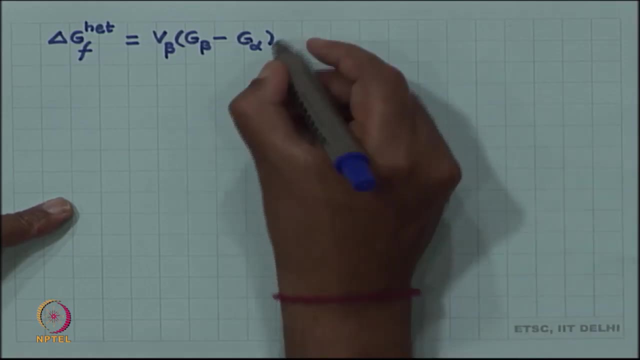 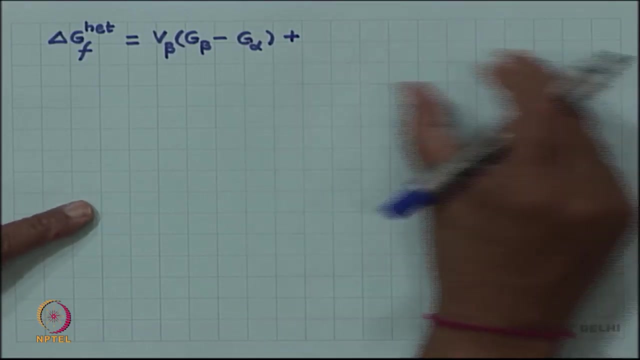 into beta. So we generated so much of free energy- V beta into g beta- but we have lost V beta into g alpha. This is the volume energy term. then we have surface energy term, and now there are three different kinds of surface energy terms, as you saw. 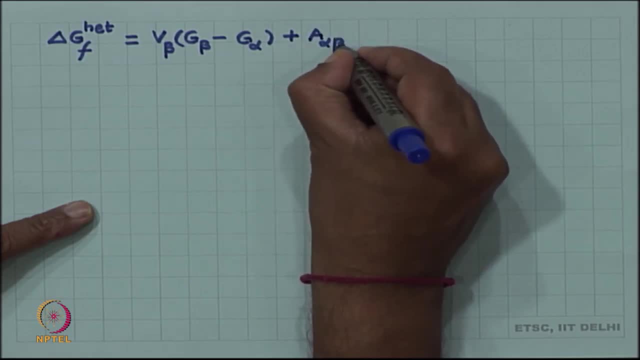 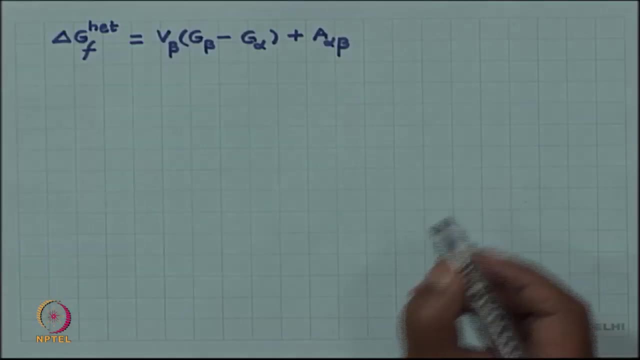 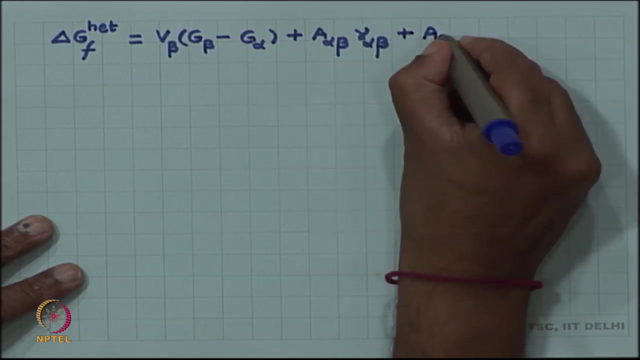 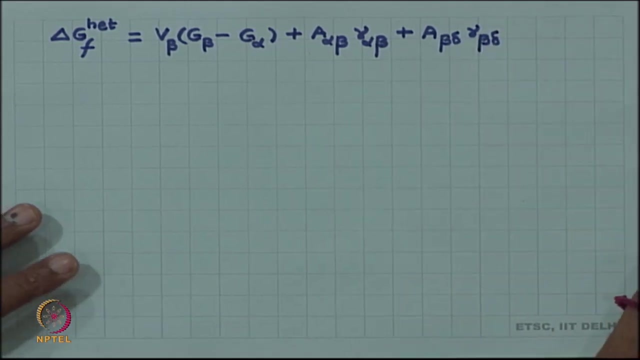 So we have A alpha beta that is the curved surface of the nucleus, that is this surface, A alpha beta times surface energy per unit area of alpha beta surface. So A alpha beta, gamma, alpha beta. we also formed the base of the nucleus, which is A beta delta, gamma beta delta. But 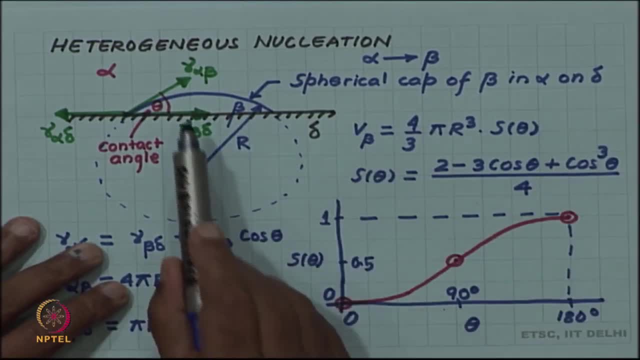 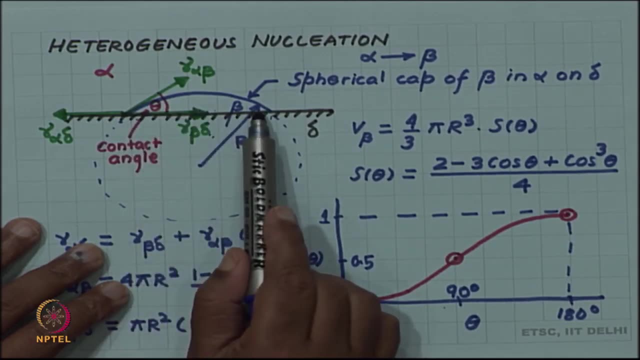 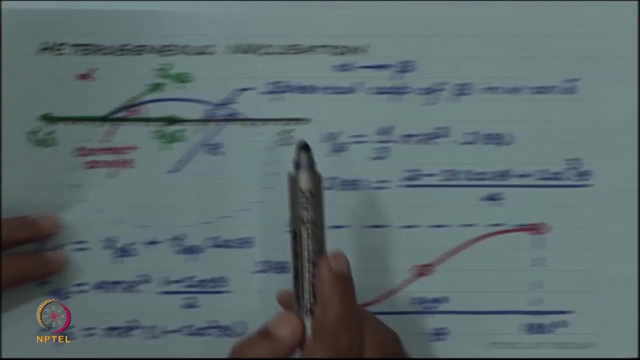 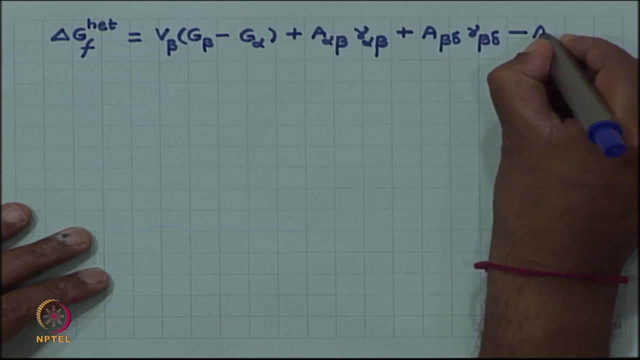 then, when we created this surface, recall that when we created this beta delta surface, due to nucleation, before nucleation, the same surface was alpha delta, because alpha was filling this entire space. So the amount of area which we created for beta delta, same amount of area was removed from alpha delta. So let me not write this as alpha delta. let me. 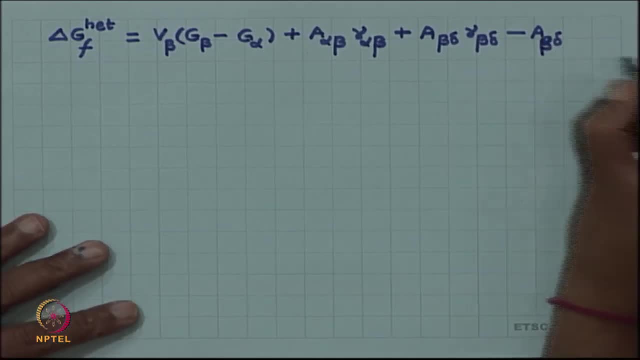 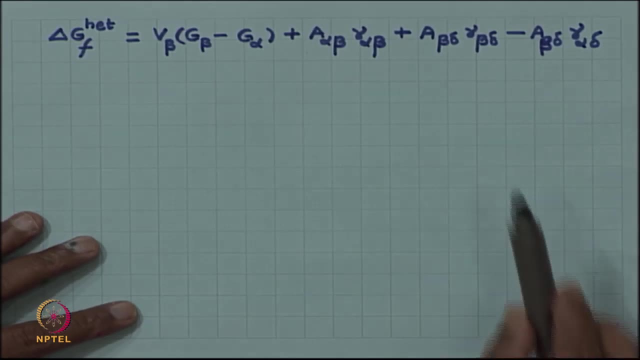 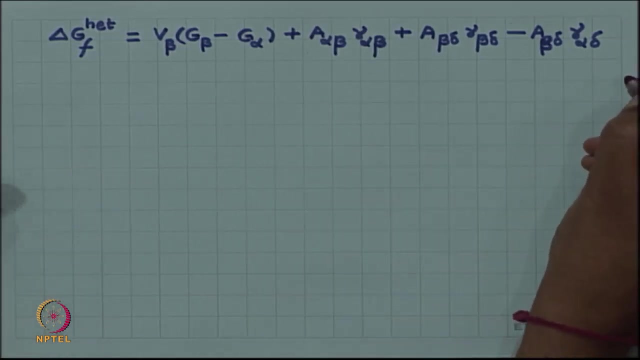 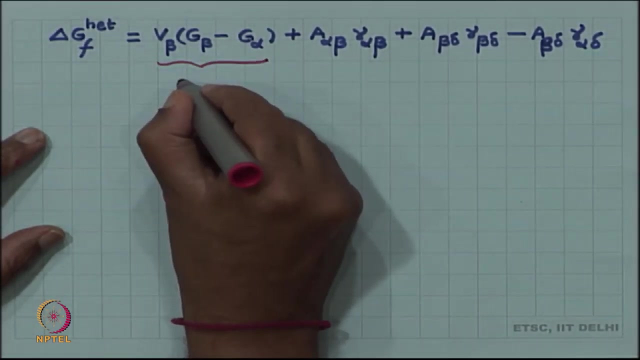 keep writing this as beta delta only, Because the area is the same, but the surface energy is alpha delta, So this is an important So recall that in homogeneous nucleation the volume energy was the driving force. So here also, volume energy is the driving force. 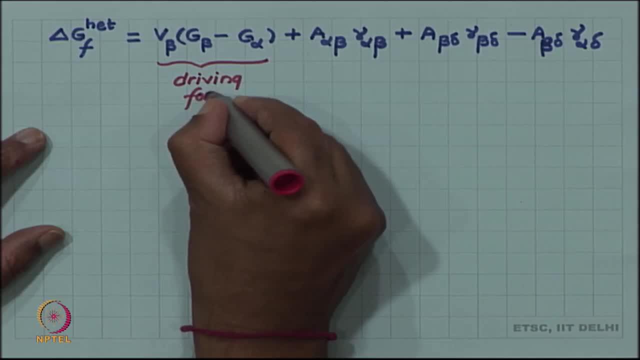 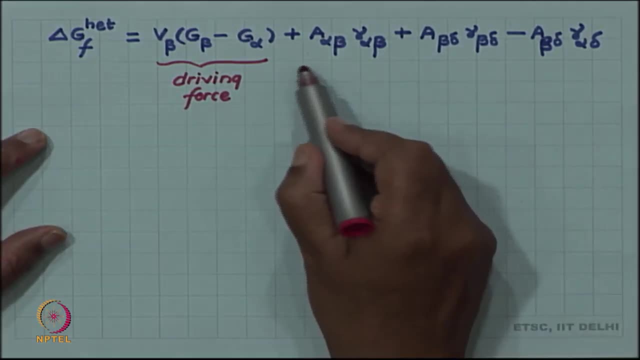 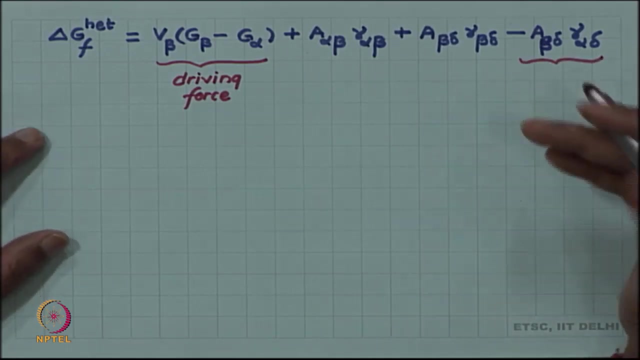 So here also volume energy is the driving force And there the surface energy was barrier to nucleation. Here also surface energy is barrier to nucleation, but one surface term. since it is getting deleted, since it is in being removed, this surface term also acts like a driving force. So there is an additional. 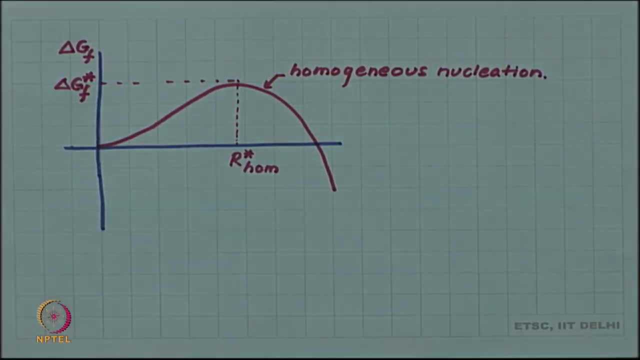 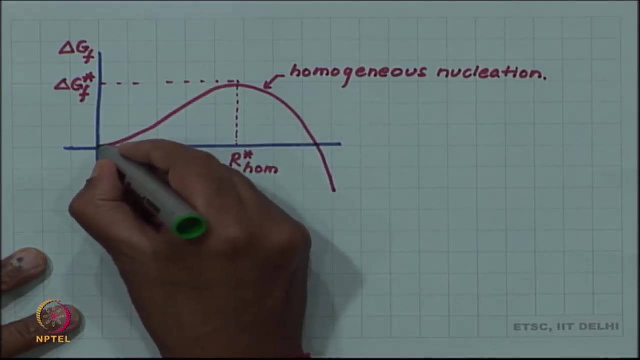 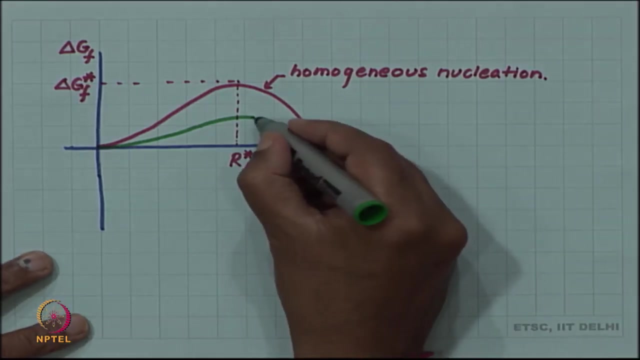 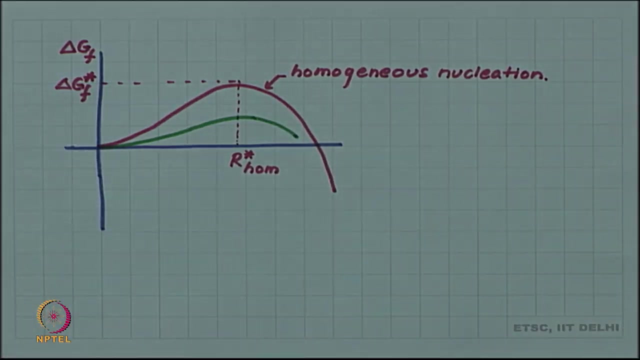 Increase the curve for heterogeneous nucleation. on these´m we found that r star is goes same. 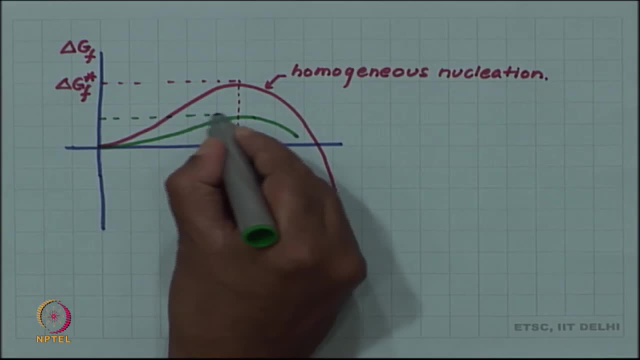 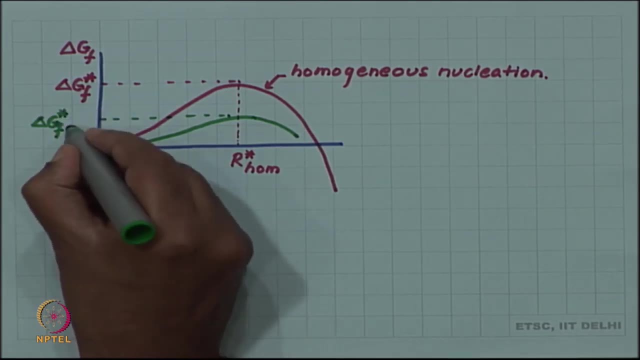 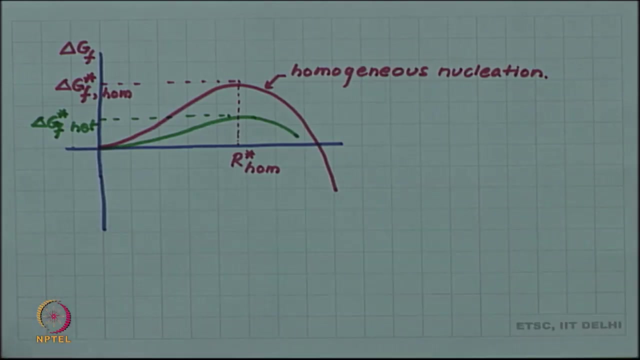 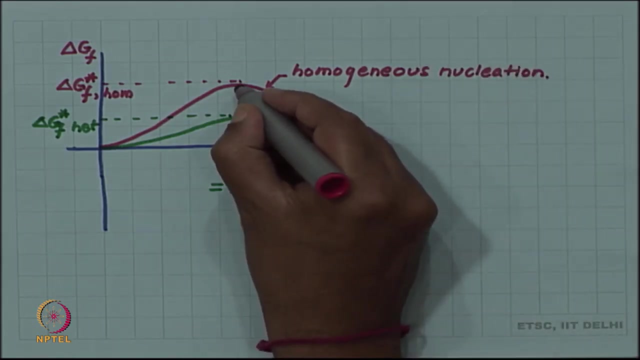 Click e also we will get the maximum at the same value for heterogeneous as well as delta g of star for homogeneous and, as we saw, r star was the same. So this is same as. So you can, you can think of this energy. initially, the energy. 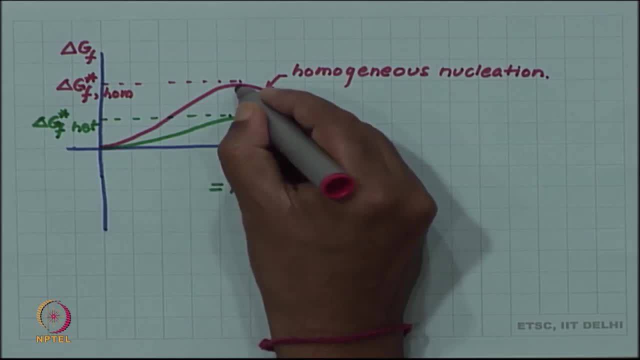 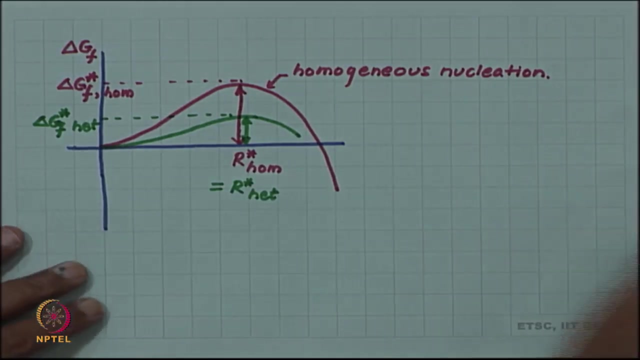 of the system has to increase. So this is a kind of energy barrier for the nucleation, and this energy barrier for nucleation also will be lower for heterogeneous nucleation. Then for the homogeneous nucleation and if you derive the expressions for these, this: 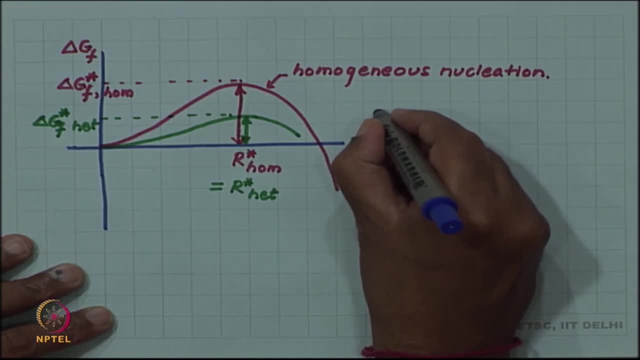 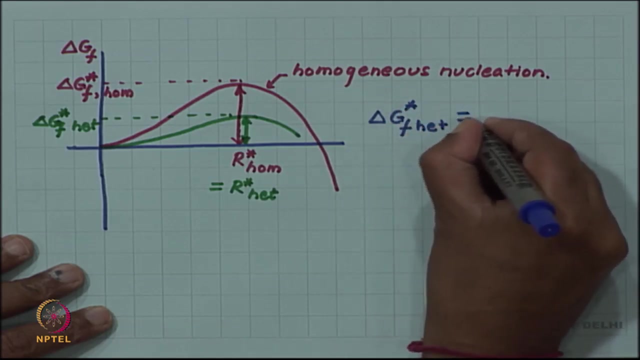 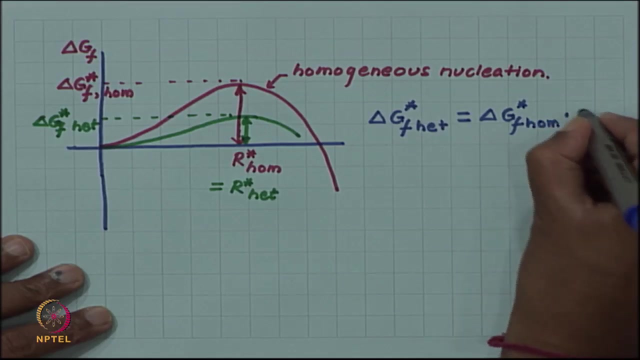 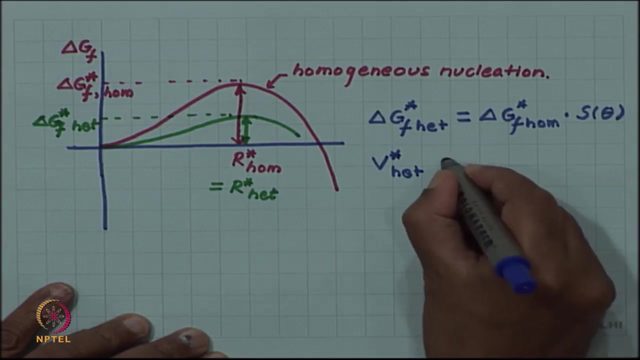 will turn out to be again, is smaller by the same factor s theta which we have been using for the volume. So delta g of star for heterogeneous is delta g of star for homogeneous. So this is the same factor s theta and we have already seen that v star for heterogeneous v star. 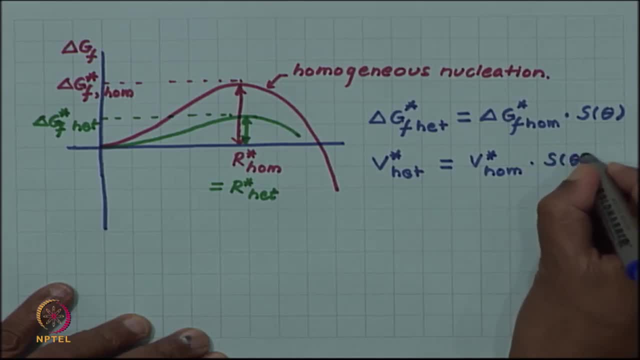 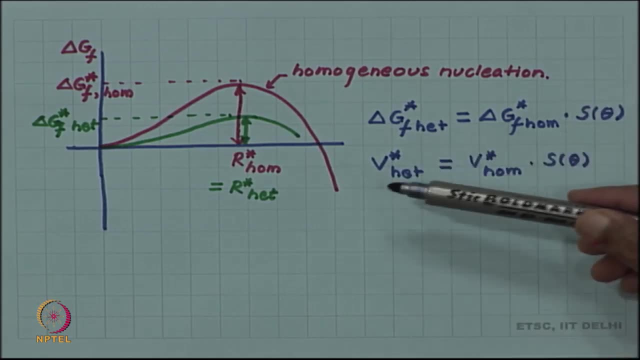 for homogeneous times s theta. So smaller is the contact angle is smaller is s theta and is volume of heterogeneous nucleus. So you have to assemble lesser number of atoms to form the heterogeneous nucleus. Similarly, the energy barrier for nucleation, that extra energy.